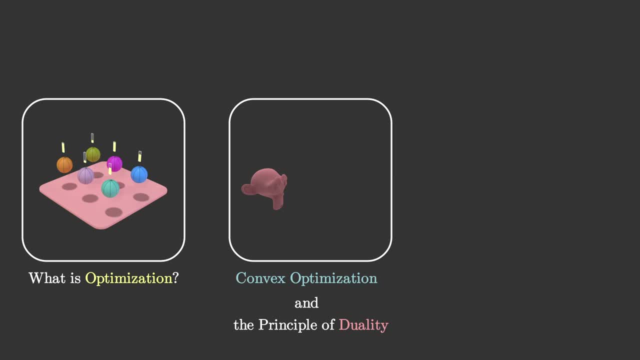 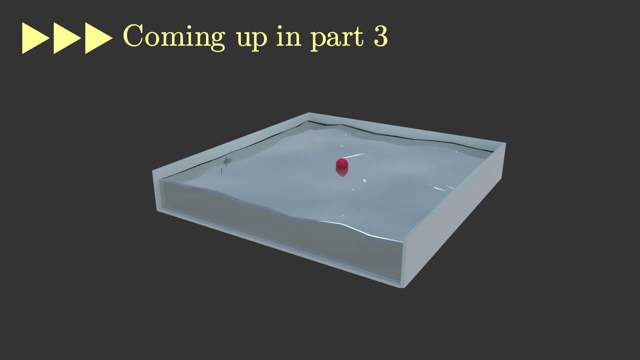 a fascinating related concept, that is, the principle of duality. The third and last part has a more algorithmic component. There we will finally have all the necessary ingredients to overview the interior point method for convex optimization. As a bonus, if you stick around until the end, you will know what this ocean animation. 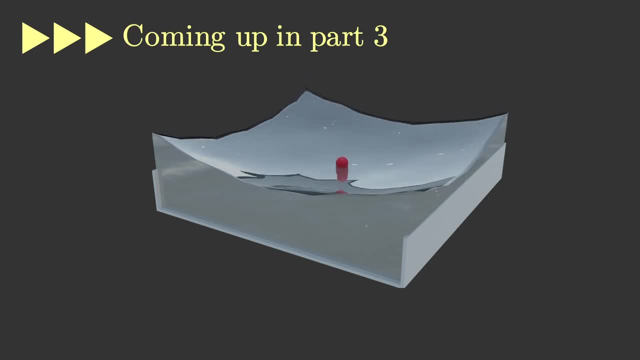 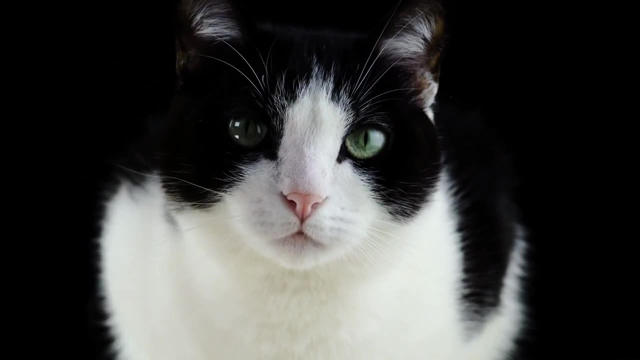 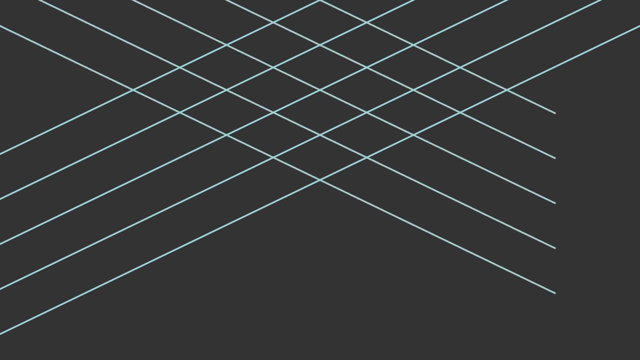 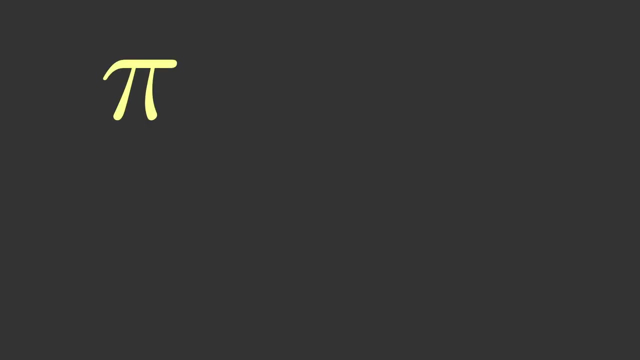 represents and how it relates to the topic of optimization. This video series is intended for anyone who is curious about mathematics and its applications. It should be accessible to a wide range of audiences. since it does not require any specific background beyond basic linear algebra and basic calculus, It is suited for math and 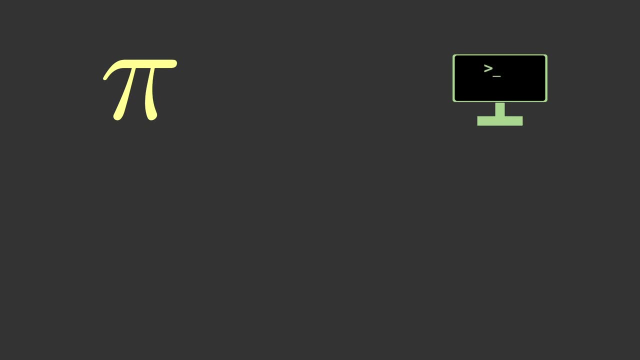 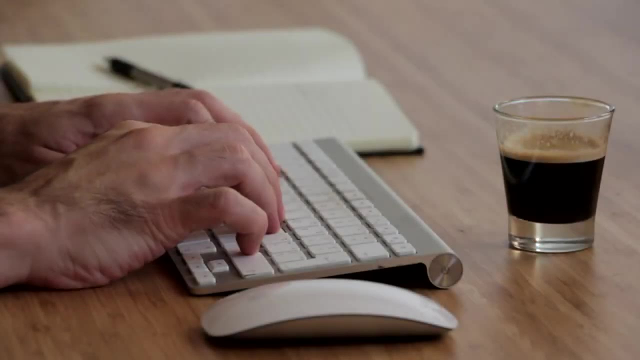 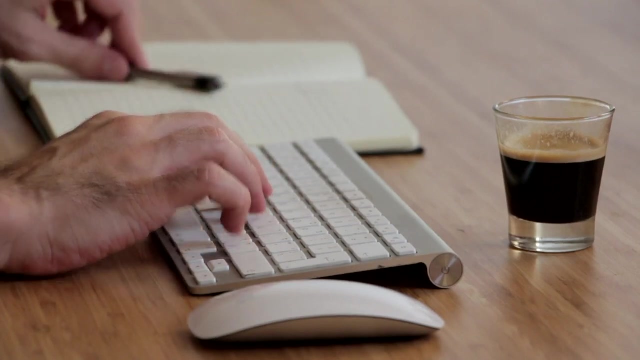 computer science students who want to know more about optimization, but also researchers or engineers who might have heard of optimization before and want to know what they can gain from it or how they can use it in their own work or research projects. Let me point out here that these videos represent my personal take on the topic of convex optimization. 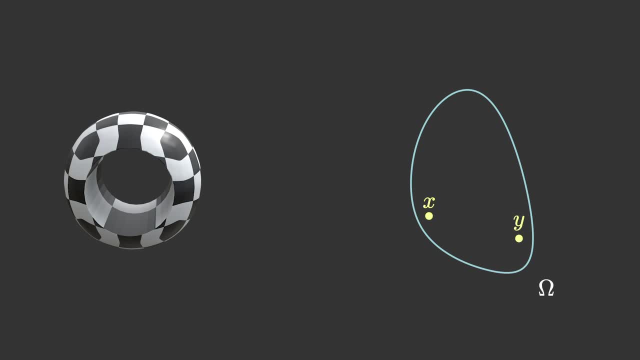 so it might be a little different from more traditional expositions that you might find elsewhere, And it is by no means exhaustive, but my goal here is to give a self-contained presentation that is crisp, visual and focuses on building intuition without getting bogged down with. 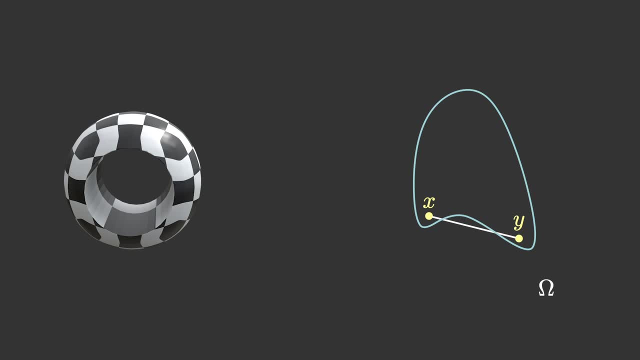 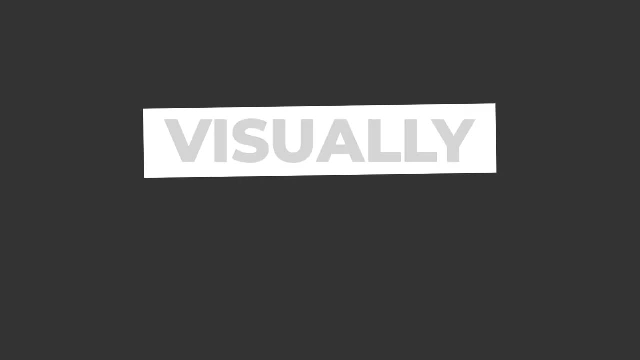 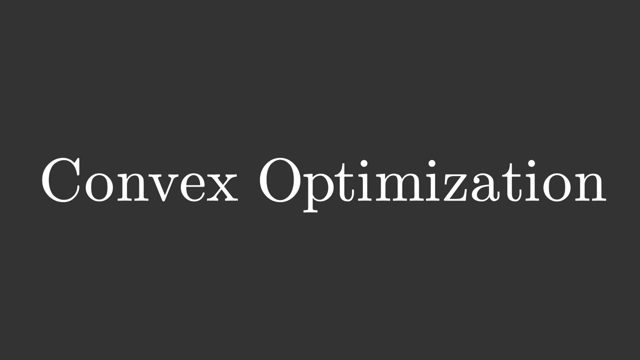 too much mathematical details, which you can always check later if needed. And with that being said, it's time to grab some coffee, because we're about to get started. Before we talk about convex optimization, let's take a step back. 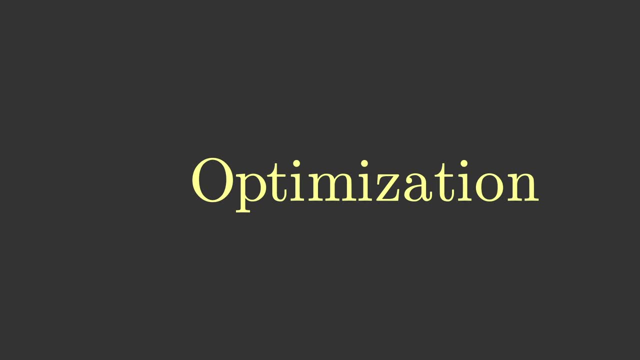 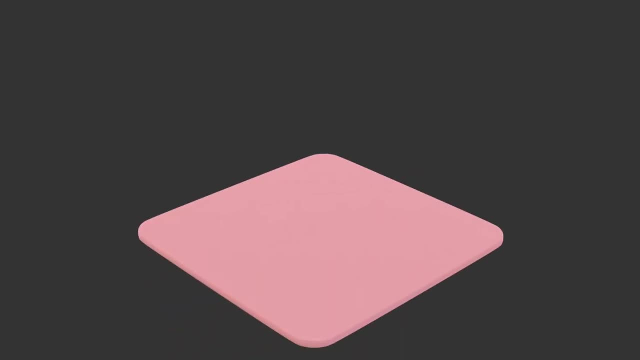 Let's first define optimization. What do we mean when we refer to some problem as an optimization problem? Well, you have an optimization problem whenever you are faced with a bunch of options that you can choose from, where each option has a cost associated with it and your job is. 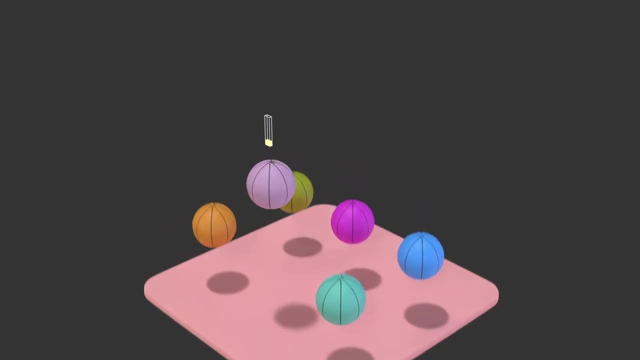 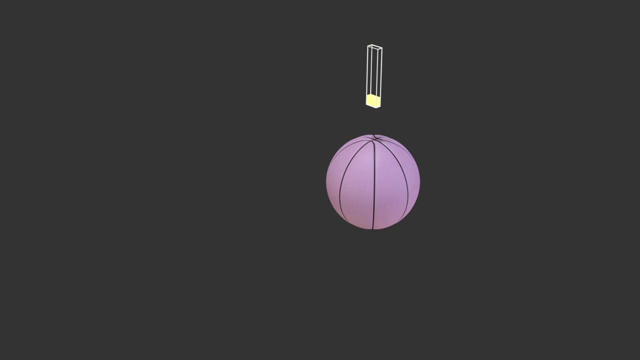 to make the optimal choice, or, in other words, you need to pick the option with the smallest possible cost. Note that sometimes in optimization, there are situations where we want to pick the option which maximizes some given metric, often referred to as a reward, rather than minimize a cost. 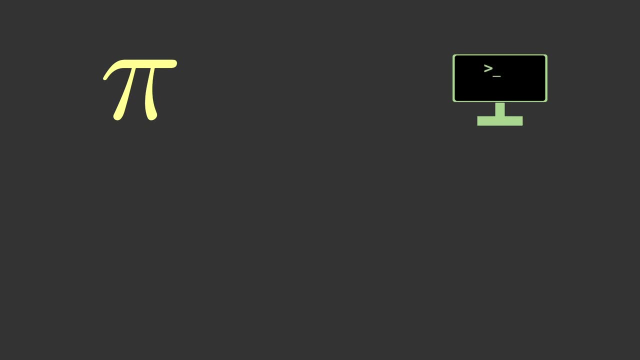 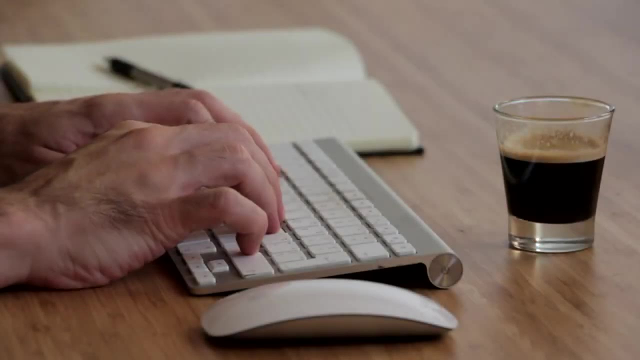 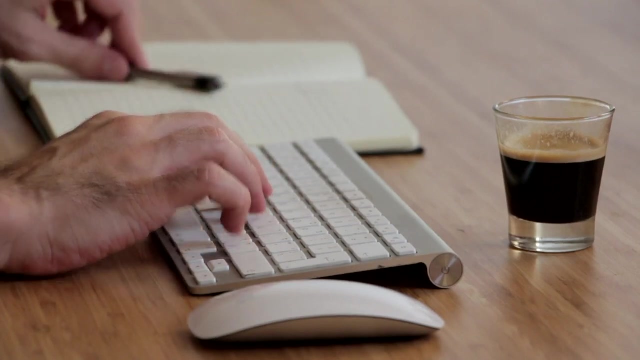 computer science students who want to know more about optimization, but also researchers or engineers who might have heard of optimization before and want to know what they can gain from it or how they can use it in their own work or research projects. Let me point out here that these videos represent my personal take on the topic of convex optimization. 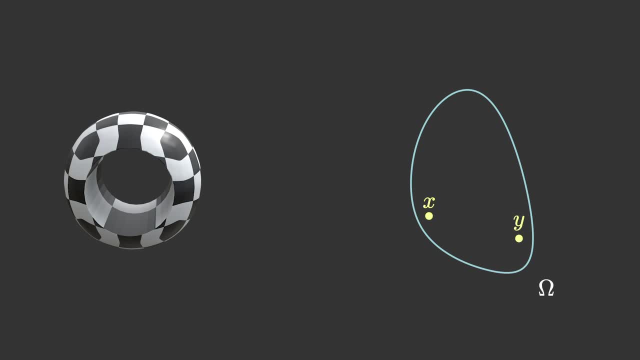 so it might be a little different from more traditional expositions that you might find elsewhere, And it is by no means exhaustive, but my goal here is to give a self-contained presentation that is crisp, visual and focuses on building intuition without getting bogged down with. 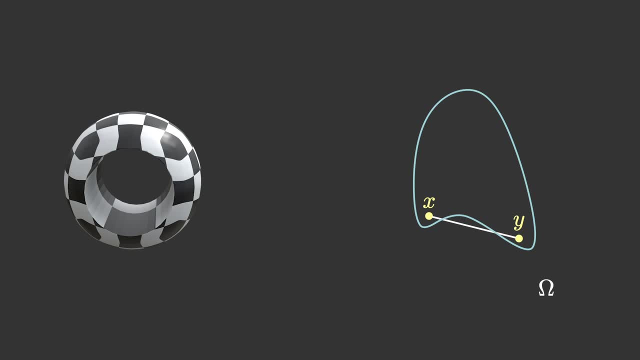 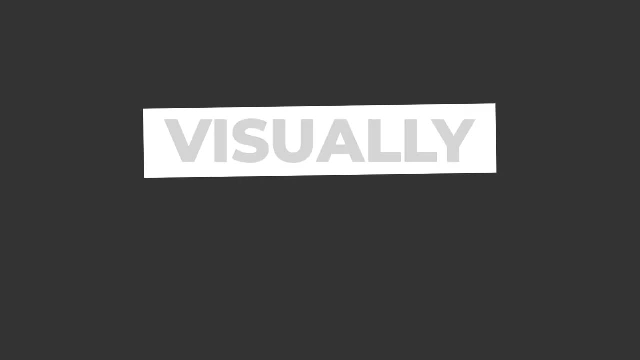 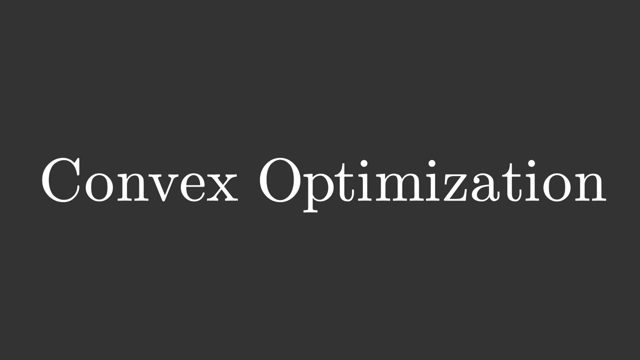 too much mathematical details, which you can always check later if needed. And with that being said, it's time to grab some coffee, because we're about to get started. Before we talk about convex optimization, let's take a step back. 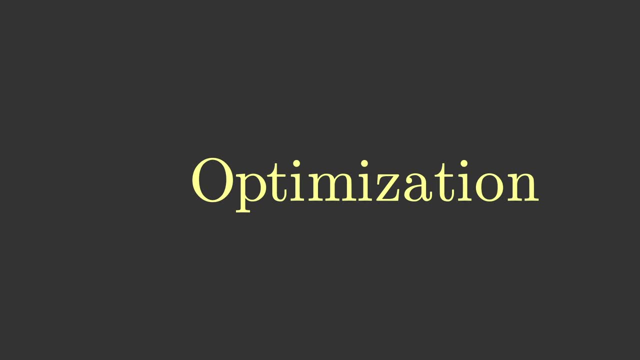 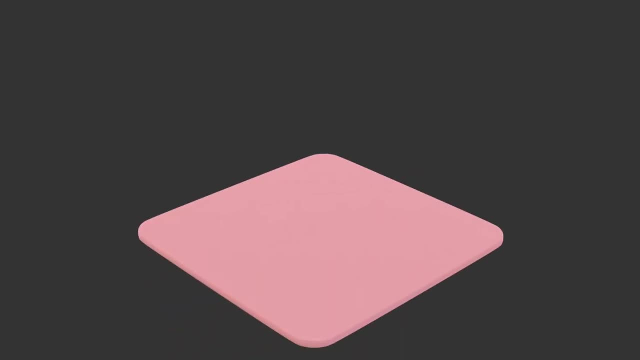 Let's first define optimization. What do we mean when we refer to some problem as an optimization problem? Well, you have an optimization problem whenever you are faced with a bunch of options that you can choose from, where each option has a cost associated with it and your job is. 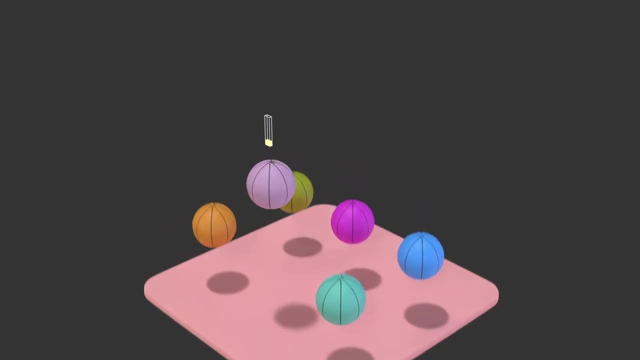 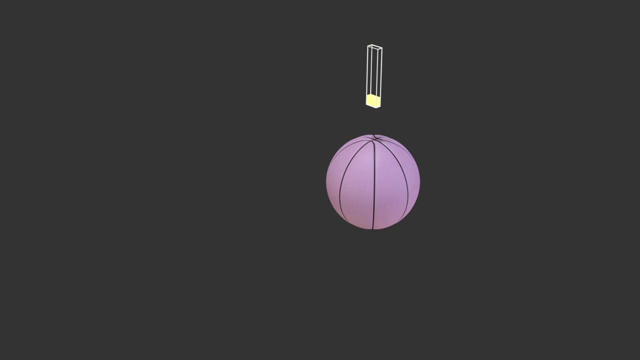 to make the optimal choice, or, in other words, you need to pick the option with the smallest possible cost. Note that sometimes in optimization, there are situations where we want to pick the option which maximizes some given metric, often referred to as a reward, rather than minimize a cost. 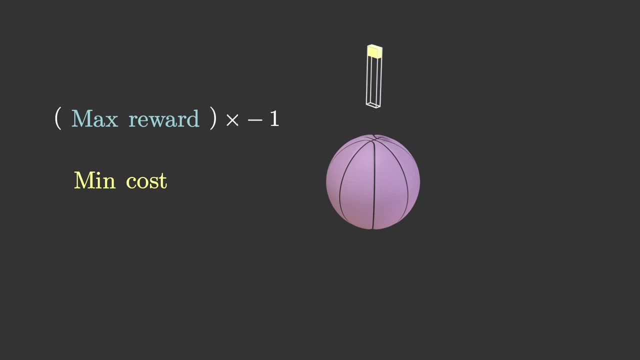 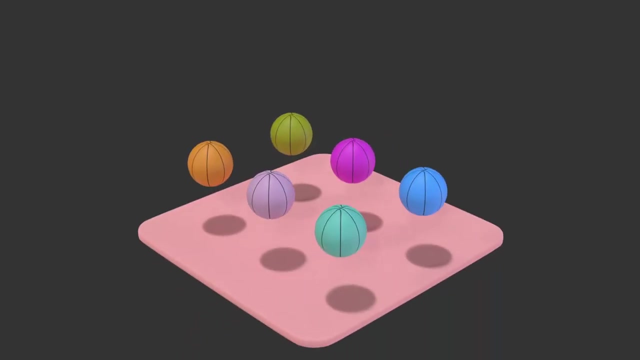 Without loss of generality. we can simply multiply the reward by minus one and convert a maximization problem to a minimization one. So for the rest of this video I'm going to follow a cost minimization convention. Note also that in this toy example there are only six options. 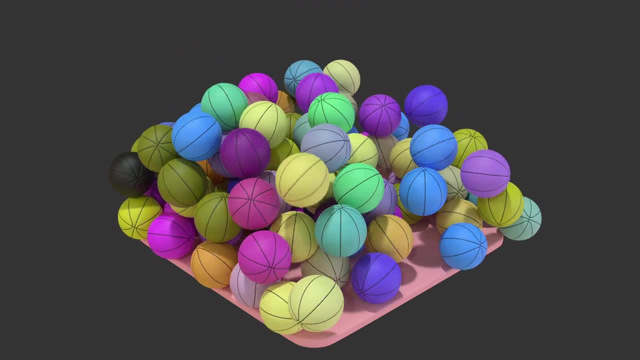 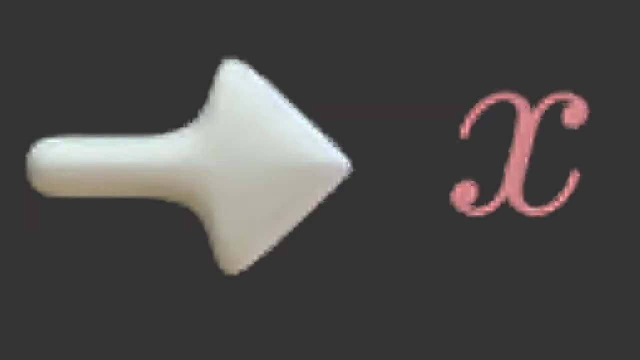 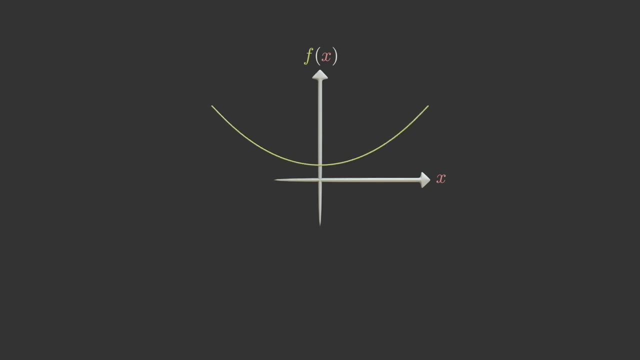 In general, however, The number of options could be huge or even infinite. A typical example where the number of options is infinite is when you try to pick a real number, x, from the continuum of all real numbers. that minimizes some given function, f. 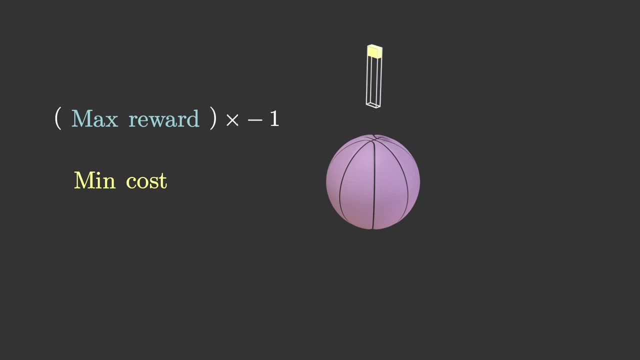 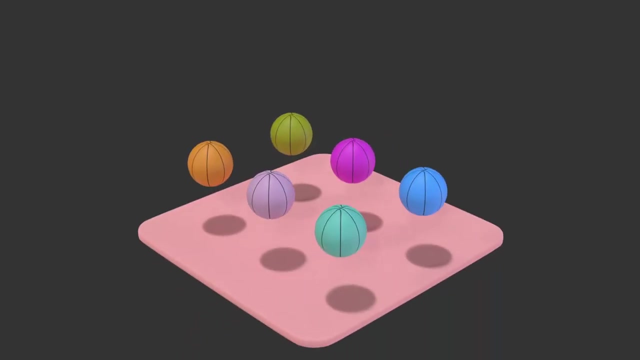 Without loss of generality. we can simply multiply the reward by minus one and convert a maximization problem to a minimization one. So for the rest of this video I'm going to follow a cost minimization convention. Note also that in this toy example there are only six options. 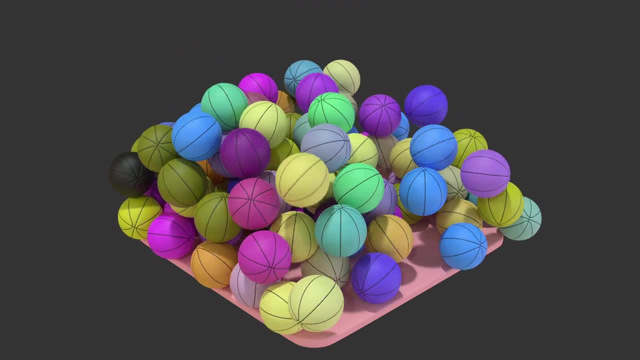 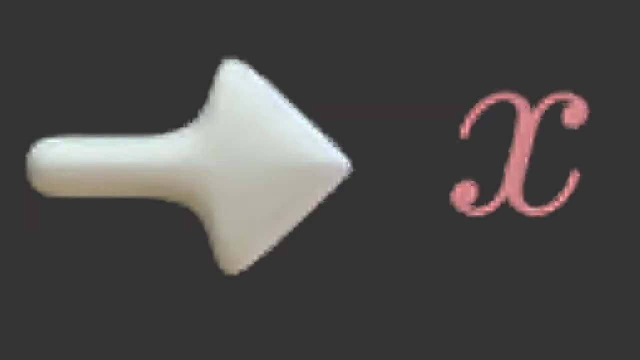 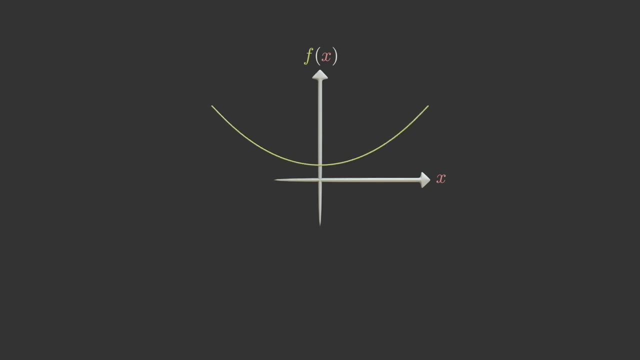 In general, however, The number of options could be huge or even infinite. A typical example where the number of options is infinite is when you try to pick a real number, x, from the continuum of all real numbers. that minimizes some given function, f. 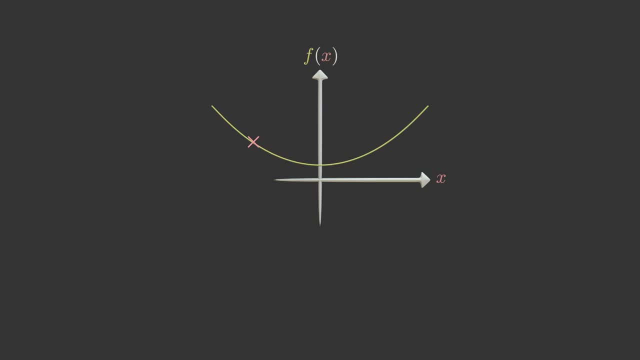 Said differently. you try to pick a scalar, x that we refer to as a decision variable, such that f is as small as possible. Here x is a one-dimensional scalar, but it could also be multidimensional. For example, x could be a two-dimensional vector, x1, x2, a three-dimensional vector. 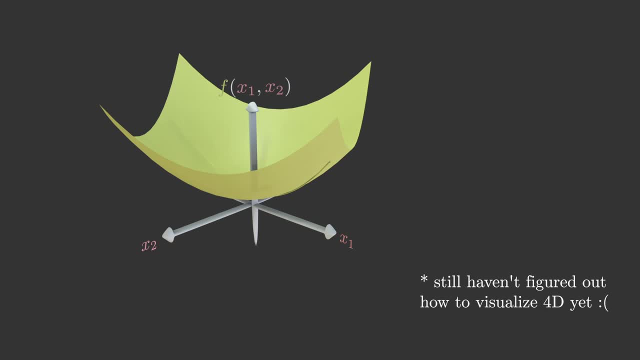 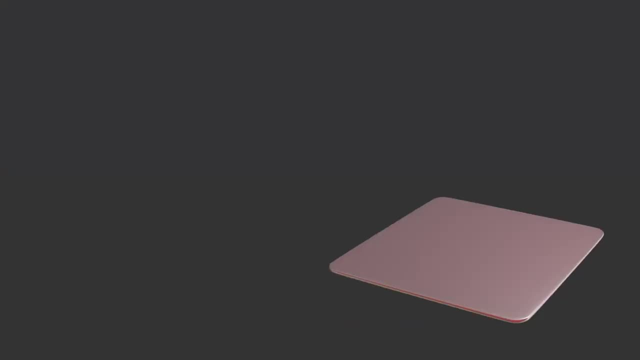 x1,, x2,, x3, etc. More formally, an optimization problem is given by three ingredients. The first ingredient is a set where our decision variable lives. Often this is simply rm. The second ingredient is a cost function, f, that we want to minimize. 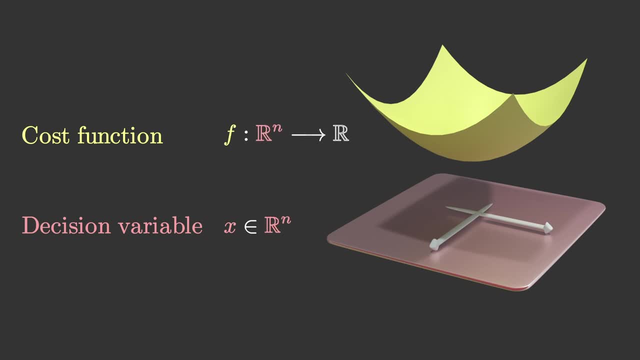 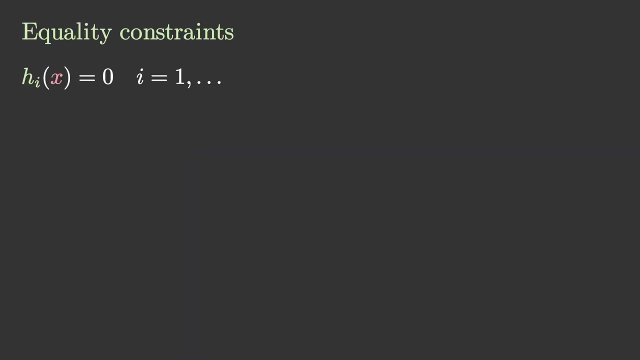 This function maps the set where our decision variable lives to r. This function is sometimes known as the objective function. The third and final ingredient are constraints on the decision variable. Constraints come in the form of equality constraints and inequality constraints. The equality and inequality constraints are two things. 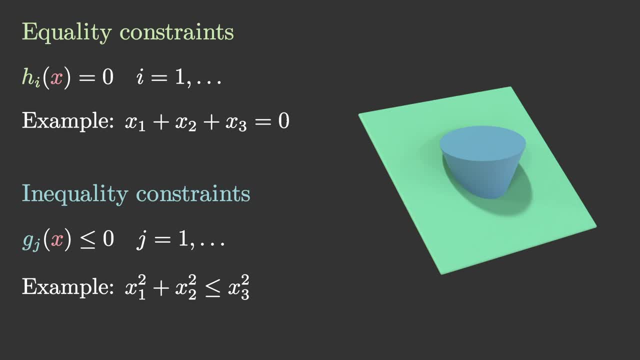 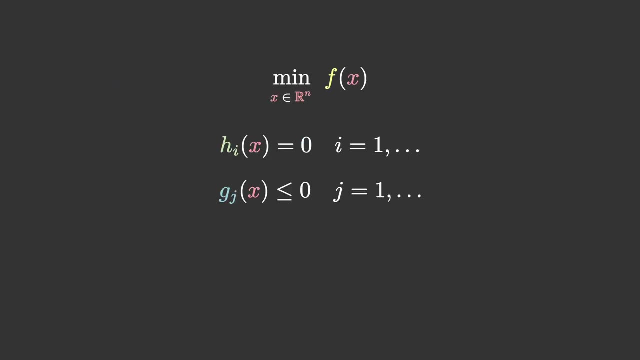 First, we take the equality constraint, We create a value, We call it the function constraints. together define what is known as the feasible set or the set of possibilities where you can pick the decision variable X from. To recap, optimization problems are often written in this form. Let us right away see some. 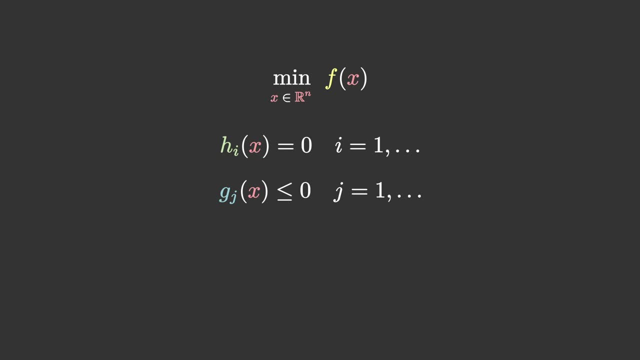 examples, When the cost function, f, is a linear function and when the functions h, i and g, j that define the constraints are linear functions as well. then we have what is known as a linear program. Linear programs are among the problems that we understand the best and, as we will see later on, it is essential to 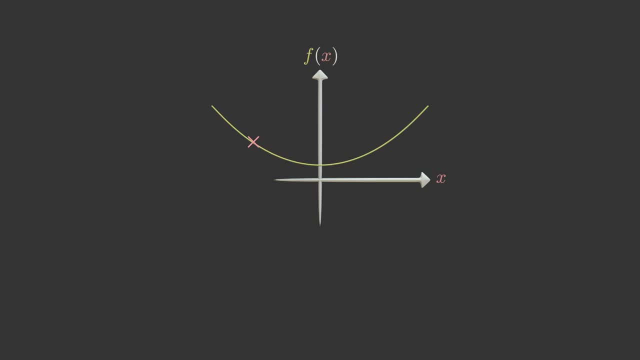 Said differently. you try to pick a scalar, x that we refer to as a decision variable, such that f is as small as possible. Here x is a one-dimensional scalar, but it could also be multidimensional. For example, x could be a two-dimensional vector, x1, x2, a three-dimensional vector. 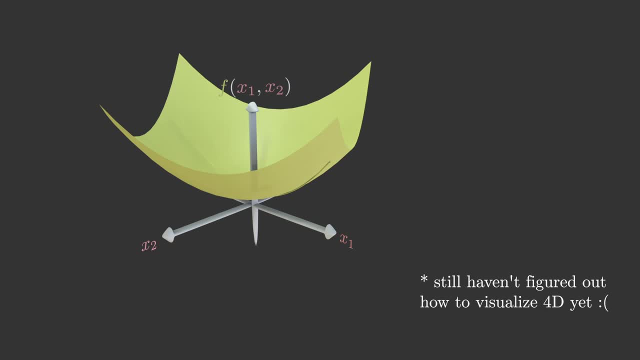 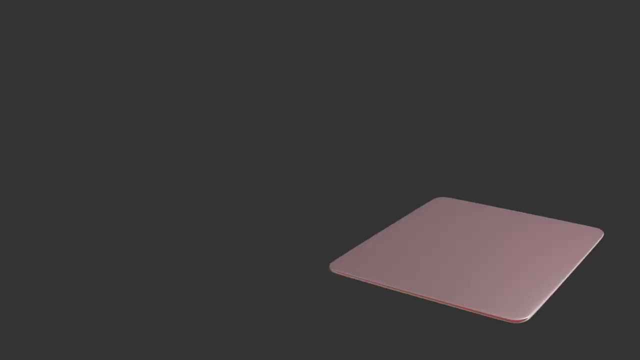 x1,, x2,, x3, etc. More formally, an optimization problem is given by three ingredients. The first ingredient is a set where our decision variable lives. Often this is simply rm. The second ingredient is a cost function, f, that we want to minimize. 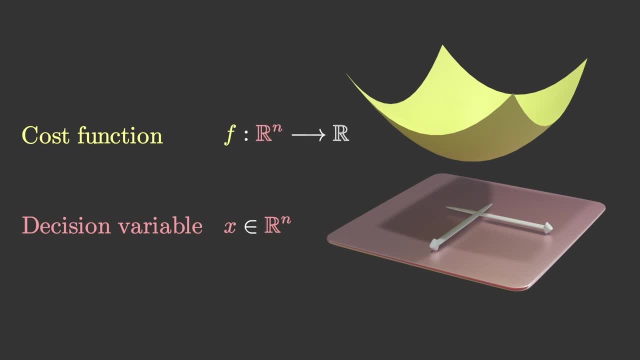 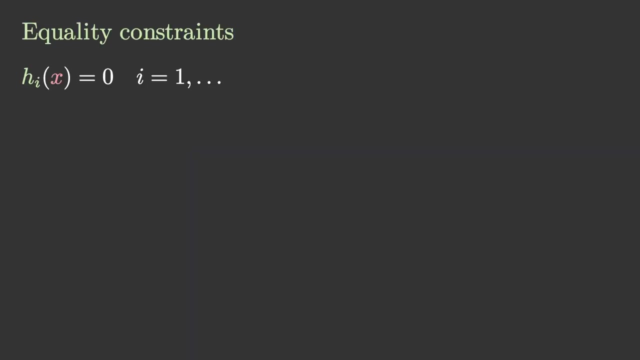 This function maps the set where our decision variable lives to r. This function is sometimes known as the objective function. The third and final ingredients are constraints on the decision variable. Constraints come in the form of equality constraints and inequality constraints. What are the constraints? 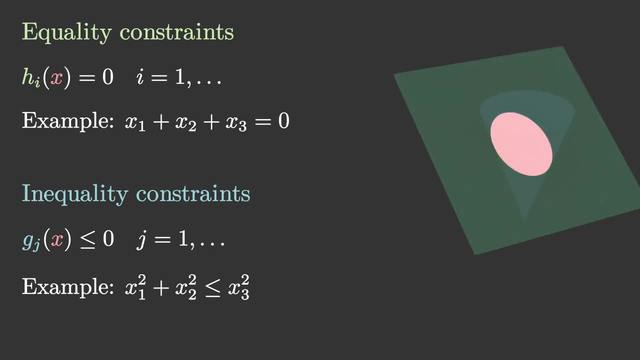 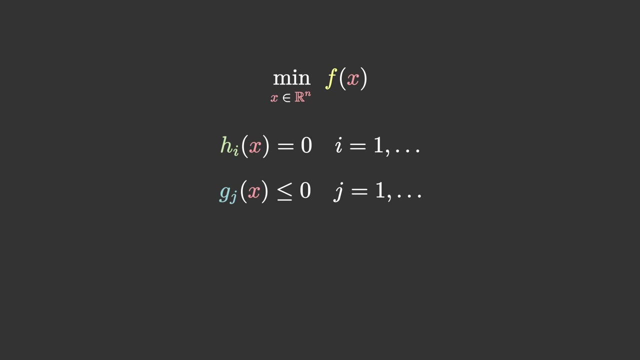 The equality and inequality constraints together define what is known as the feasible set or the set of possibilities, where you can pick the decision variable x from. To recap, optimization problems are often written in this form. Let us right away see some examples: When the cost function f is a linear function and when the functions hi and gj that define 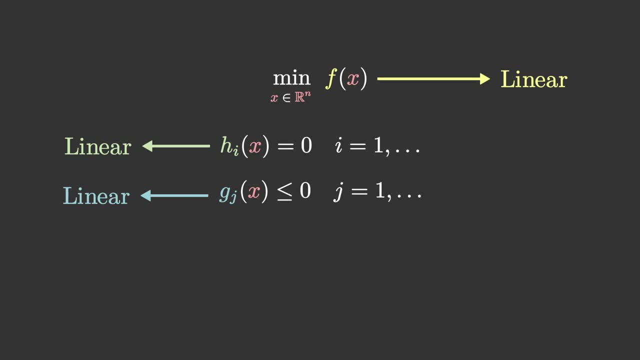 the constraints are linear functions as well. then we have what is known as a linear function. Linear programs are among the problems that we understand the best, And, as we will see later on, it is essential to understand what happens in the simpler and maybe idealistic linear world before we move on to more complicated non-linear problems. 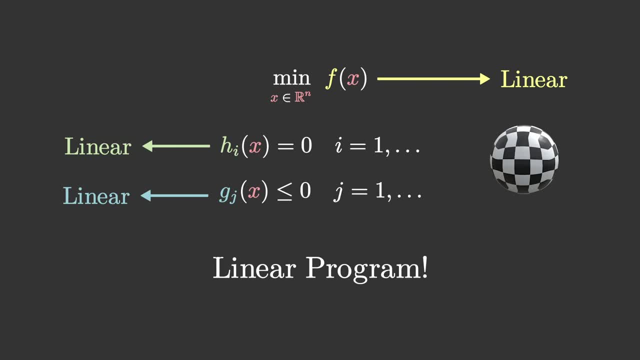 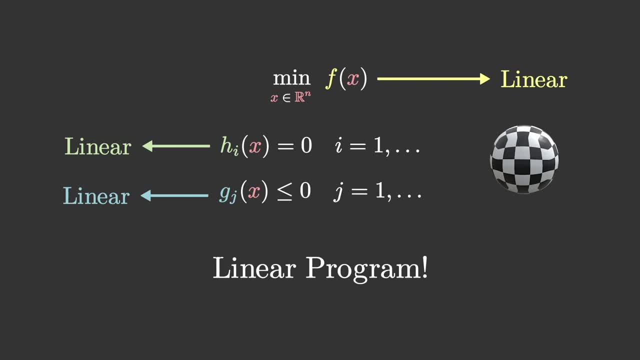 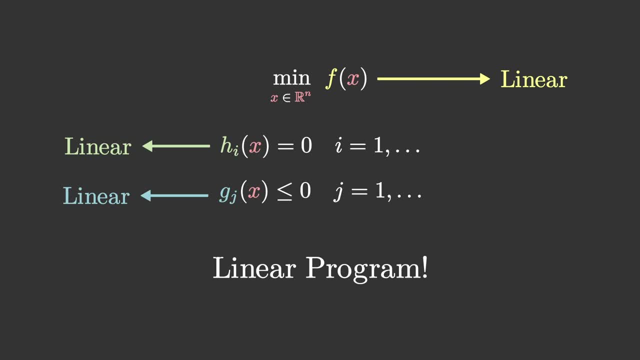 understand what happens in the simpler and maybe idealistic linear world before we move on to more complicated nonlinear problems. So in the next three minutes or so let us try to build some geometric intuition about linear programs. To visualize linear programs geometrically we need to first understand how to visualize linear functions. There are 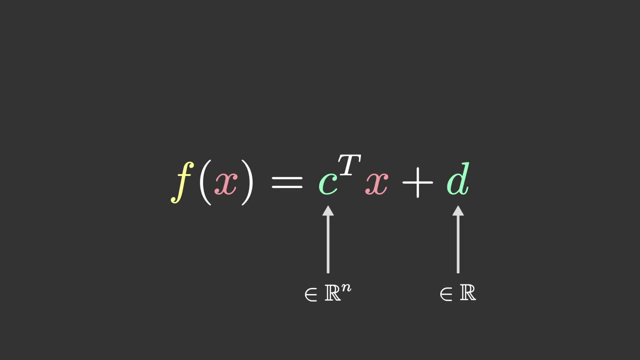 essentially two ways we could go about visualizing a linear function like this one. Either we represent it with a hyperplane with equation f of x equals 0, or with the vector c that is normal to this hyperplane. The hyperplane representation is useful for visualizing where the linear function f takes some 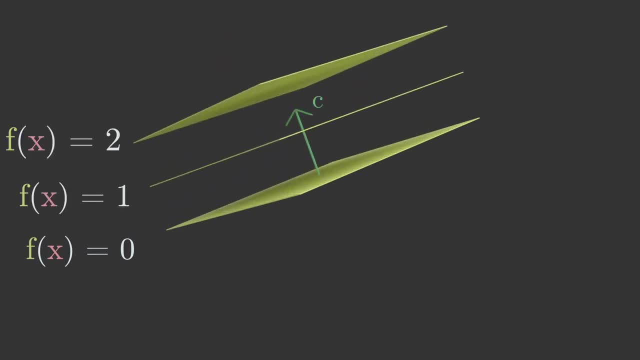 given value, like maybe f of x, equals 0,, 1 or 2.. On the other hand, the vector representation is useful for understanding the direction that increases or decreases this linear function. For linear cost functions, we prefer the vector representation. The. 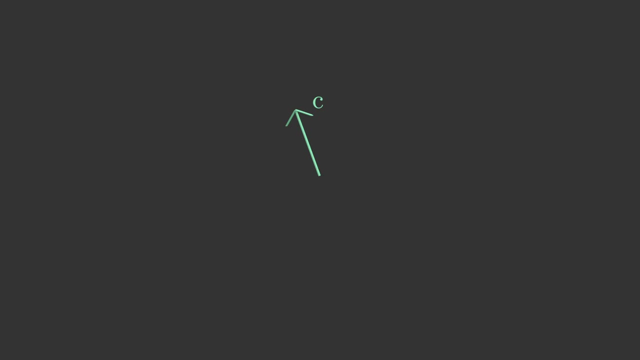 reason is that, in the absence of constraints and in order to minimize a cost, function f, what you need to do is simply move along the vector minus c as much as possible. Easy enough, So now let us see how to visualize linear constraints For linear functions that define. 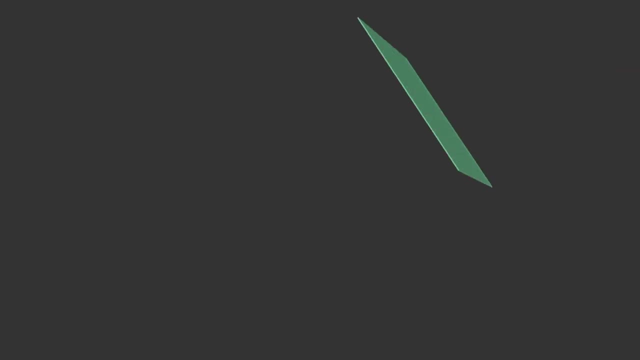 linear constraints. we prefer the hyperplane representation. A hyperplane divides the space in three regions: a positive half space, a negative half space and a null region, or the hyperplane itself. Now, if you think of the whole space, where your decision variable? 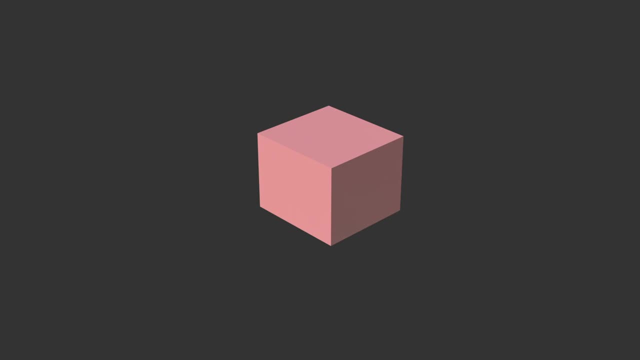 lives as this cube, then a linear constraint, for example an inequality constraint, will cut off a part of the cube. And as you add more and more linear constraints, more and more parts of the cube are going to be cut off And the region of the space that we are left with. 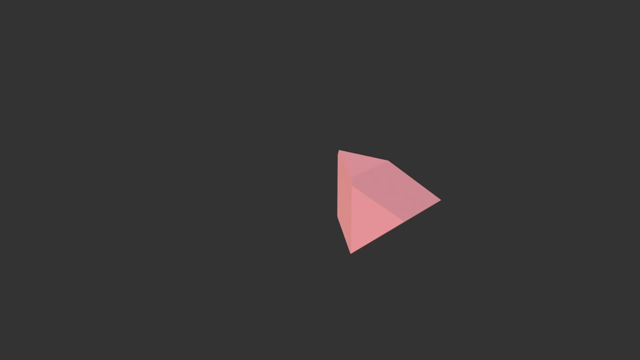 is our feasible region. Moving on, an optimization problem that might be familiar to you is linear regression or the least squares problem. Here we try to model the relationship between inputs A and outputs B And more specifically, we try to fit a linear model. So our decision variable is a vector of weight, Our objective. 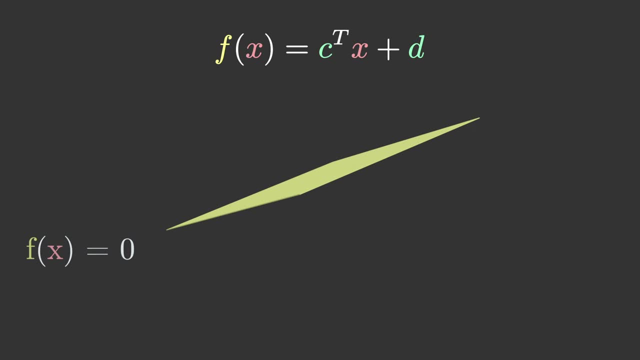 one. either we represent it with a hyperplane with equation f equals zero or with the vector c that is normal to this hyperplane. The hyperplane representation is useful for visualizing where the linear function f takes some given value, Like maybe f of x equals zero, one or z. 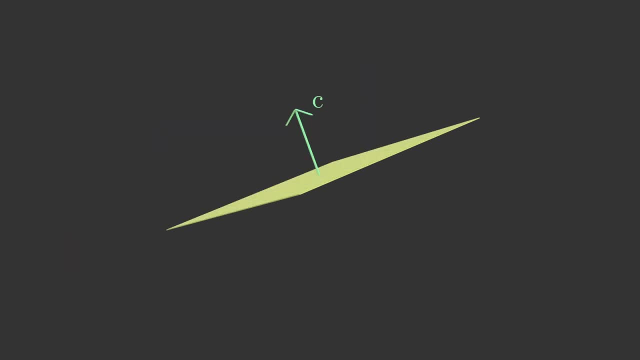 or two. On the other hand, the vector representation is useful for understanding the direction that increases or decreases this linear function. For linear cost functions, we prefer the vector representation. The reason is that, in the absence of constraints and in order to minimize a cost function f, what you need to do is: 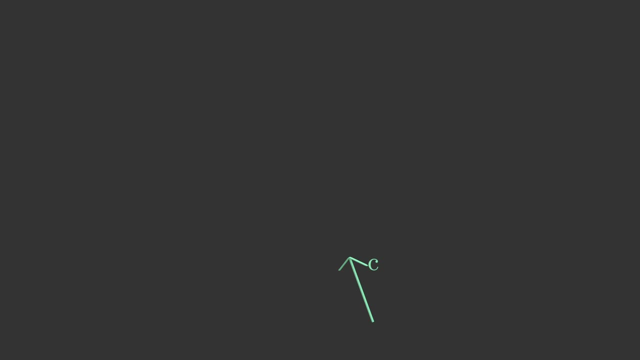 simply move along the vector minus c as much as possible. easy enough. So now let us see how to visualize linear constraints. For linear functions that define linear constraints, we prefer the hyperplane representation. A hyperplane divides the space in three regions: a positive half-space, a negative half-space. 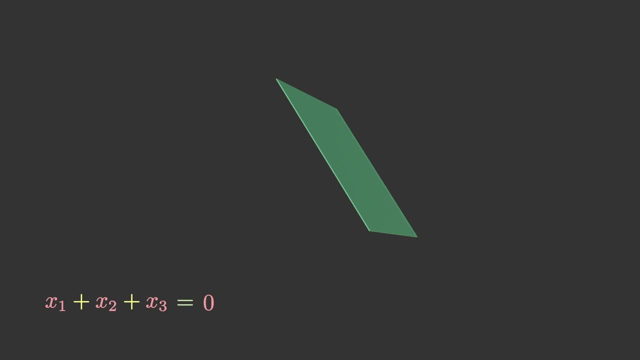 and a null region, or the hyperplane itself. Now, if you think of the whole space where your decision variable lives as this cube, then a linear constraint, for example, an inequality constraint, will cut off a part of the cube. And, as you add, 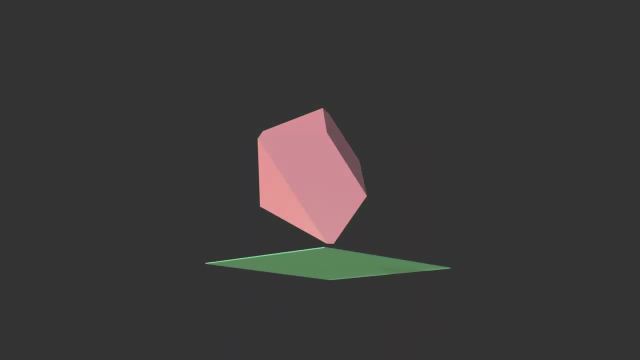 more and more linear constraints, more and more parts of the cube are going to be cut off, And the region of the space that we are left with is our feasible region. Moving on, an optimization problem that might be familiar to you is linear regression, or the least squares problem. Here we try to model the relationship. 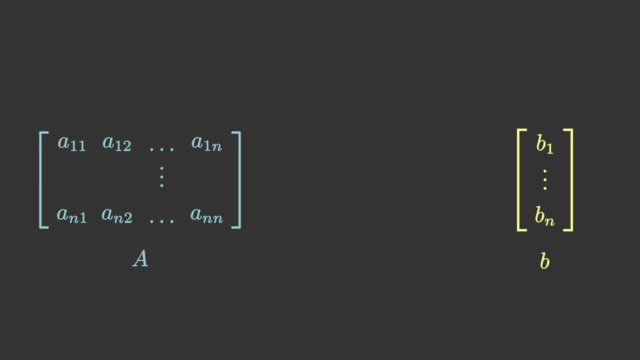 between inputs a and outputs b. More specifically, we try to fit a linear model, So our decision variable is a vector of weight. Our objective function measures the error in our linear model. And note that the objective function is not a linear function but rather a quadratic. 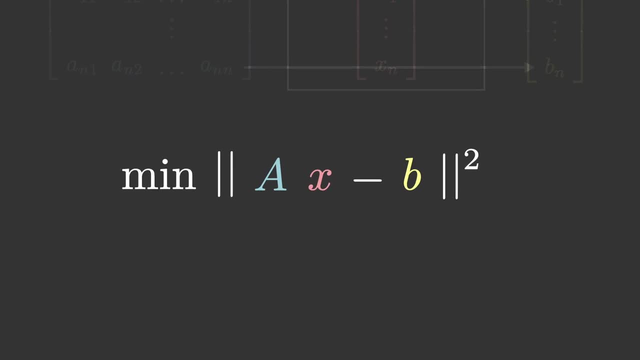 function measures the error in our linear model And note that the objective function is not a linear function but rather a quadratic function, And our constraints are. well, there aren't any constraints. example: There exists quite few variations of this problem. For example, we could replace: 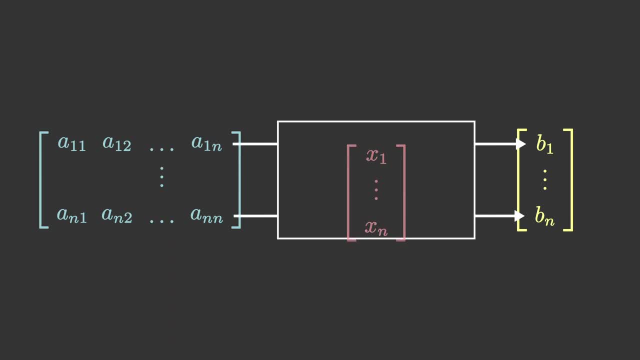 the linear model with a more complicated function like a neural network. In that case the regression problem becomes a considerably harder problem, And this should already give you a hint that some optimization problems are easier to handle than others. A third example of optimization problems I want to show you is portfolio optimization from the field of finance. In portfolio optimization, 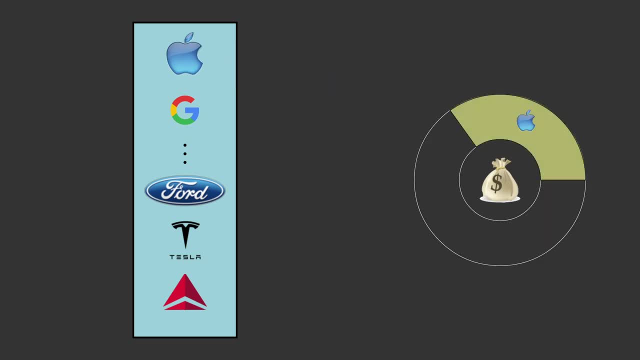 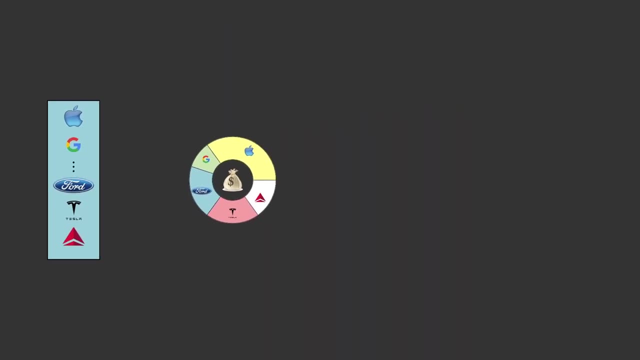 you are presented with a list of assets, like stocks, and your job is to pick which assets, and how much of each asset, you should buy. Here, your objective is to maximize returns, and your constraints are that maybe you have a fixed budget that you cannot exceed, and 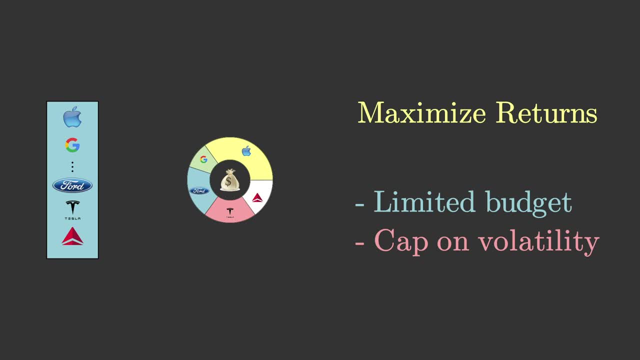 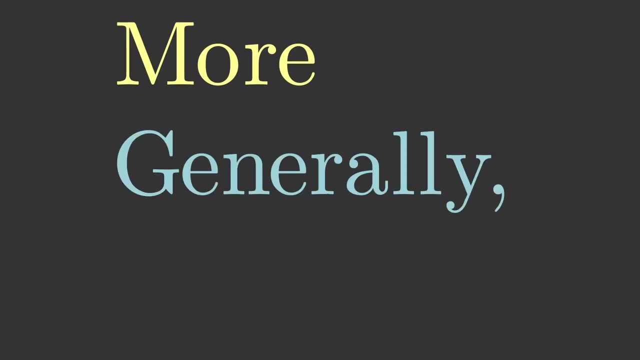 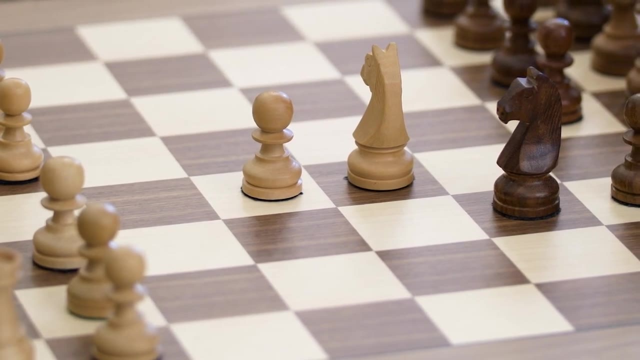 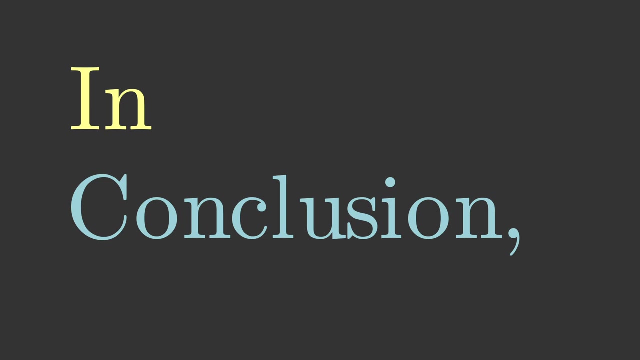 maybe you have a cap on the maximum volatility. More generally, any problem that involves taking the best decision under constraints is an optimization problem. Engineering, advertising games are just some examples. In conclusion to the first part of this series, I would like to point out that so far, we 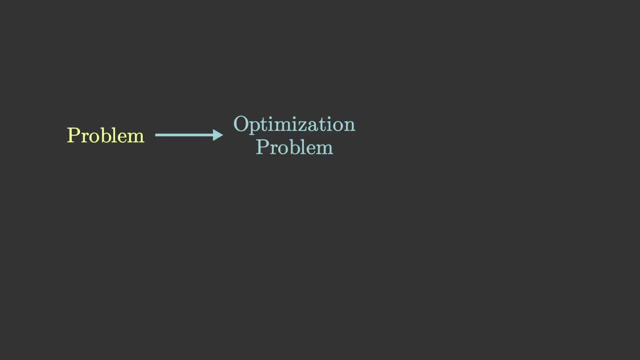 have focused on taking a problem and formulating it as an optimization problem. We have not yet discussed how you can optimize your portfolio based on the best decision you can make. In fact, optimization problems that have very similar formulations can require a completely different set of techniques to solve, and we often need to design specialized machinery. 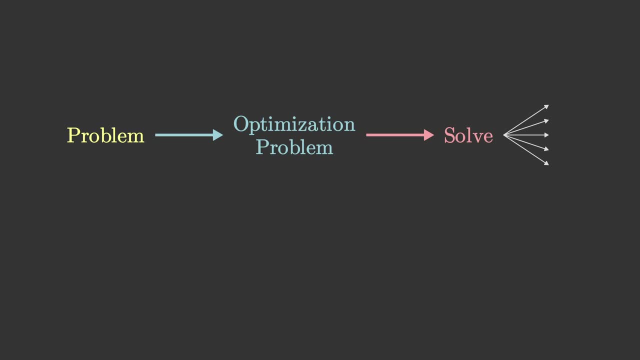 for each problem separately. In the last couple of decades, however, something magical has happened. We have discovered that a large family of optimization problems, namely convex optimization problems, are more likely to be solved by a simple combination of a set of techniques. 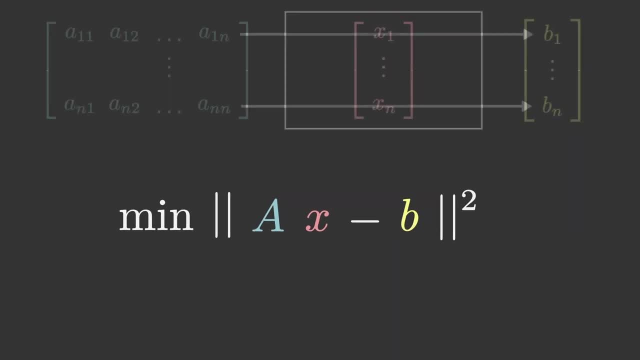 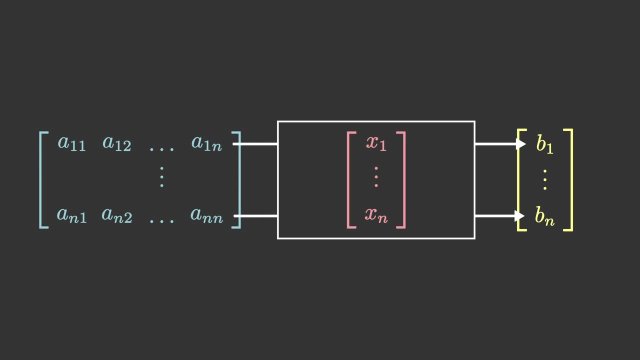 function. Our constraints are well, there aren't any constraints in this example. There exists quite few variations of this problem. For example, we could replace the linear model with a more complicated function like a neural network. In that case, the regression problem becomes a considerably harder problem. 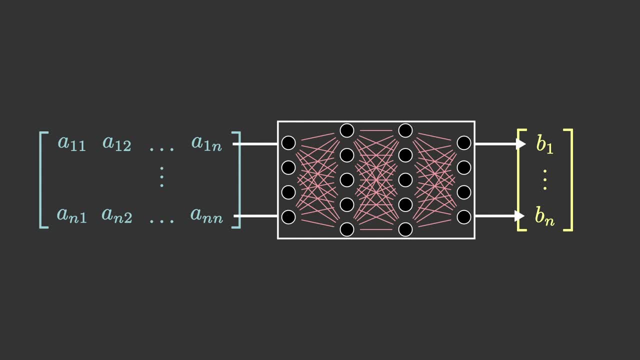 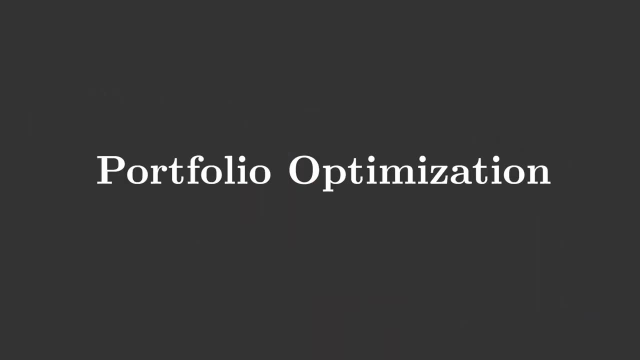 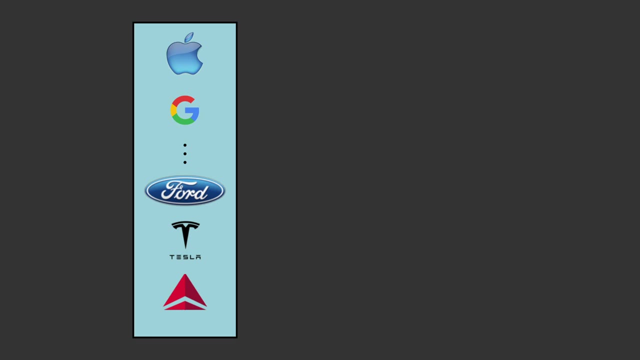 And this should already give you a hint that some optimization problems are easier to handle than others. A third example of optimization problems I want to show you is portfolio optimization from the field of finance. In portfolio optimization, you are presented with a list of assets, like stocks and your 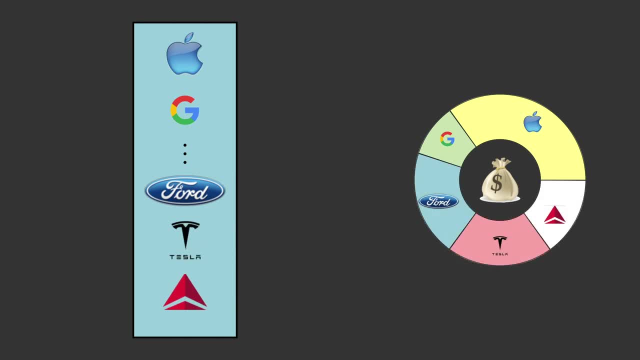 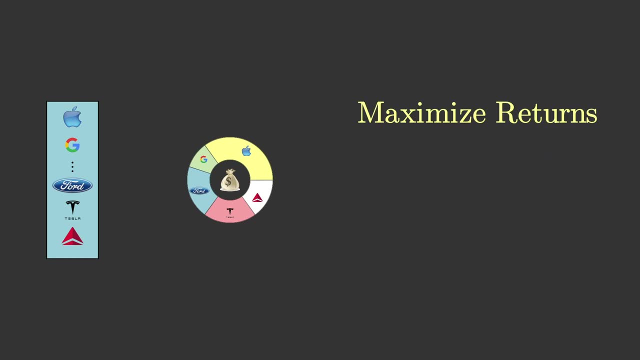 job is to pick which assets, and how much of each asset, you should buy. Here, your objective is to maximize returns, and your constraints are that maybe you have a fixed budget that you cannot handle And maybe you have a cap on the maximum volatility allowed for your portfolio. 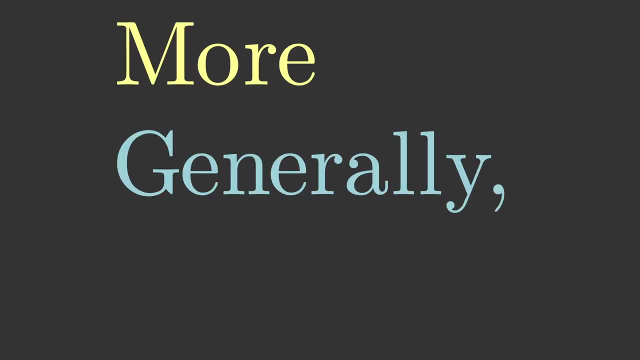 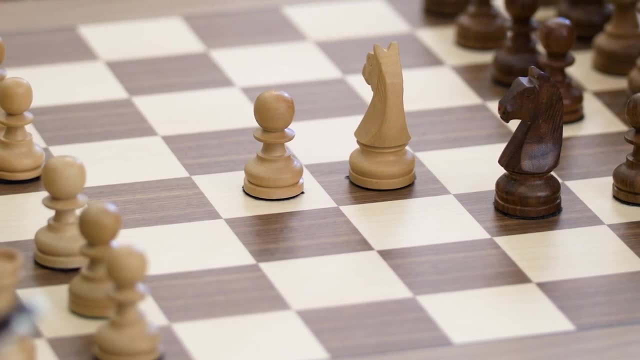 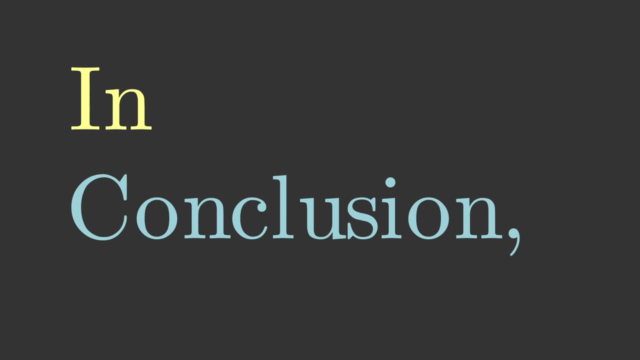 More generally, any problem that involves taking the best decision under constraints is an optimization problem. Engineering, advertising games are just some examples. In conclusion to the first part of this series, I would like to point out that so far, we have focused on taking a problem and formulating it. 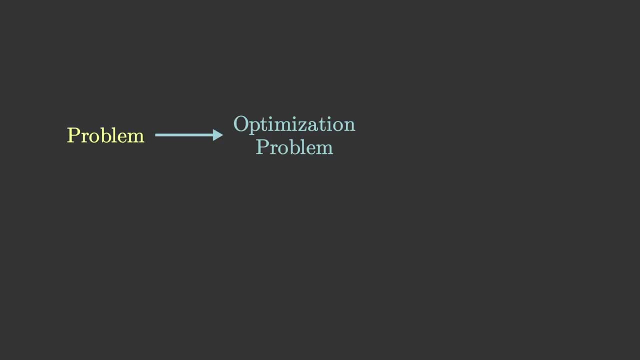 And we are not going to go into too much detail on this. We have not yet discussed how you can actually solve these problems. In fact, optimization problems that have very similar formulations can require a completely different set of techniques to solve, and we often need to design specialized machinery. 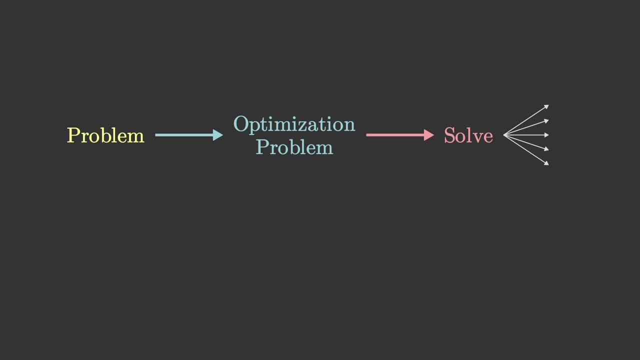 for each problem separately. In the last couple of decades, however, something magical has happened. We have discovered that a large family of optimization problems have been created, and we have been able to solve them in a unique way, Namely convex. optimization problems can be solved efficiently in a unified manner. 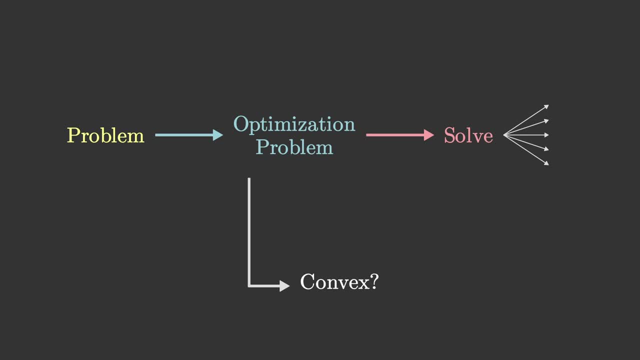 Once you recognize a given optimization problem as convex, then you can apply an already established and mature technology that people have developed for convex problems, almost as a black box. In the next video we will discuss convexity in more details and see what makes this property.